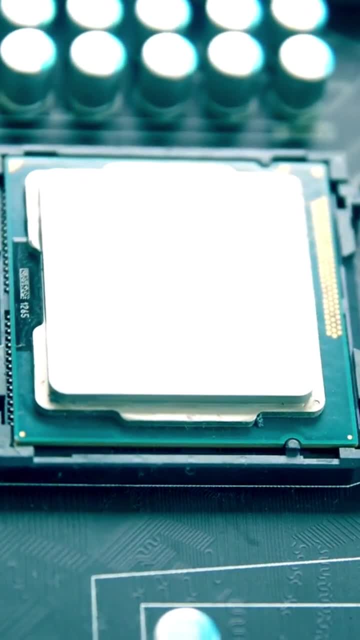 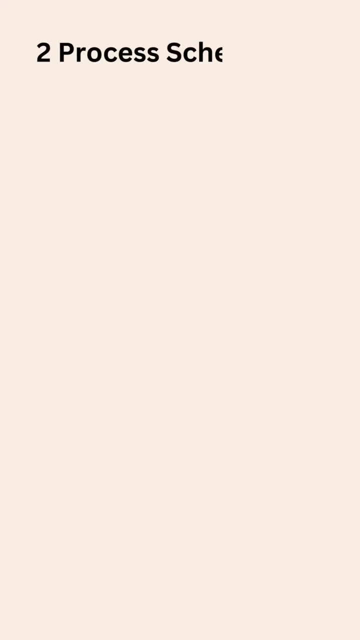 program. in execution, The process is assigned essential resources such as memory space and CPU time. 2. Process scheduling: The operating system determines the order in which processes are executed on the CPU. known as scheduling, Various scheduling algorithms, such as first-come. 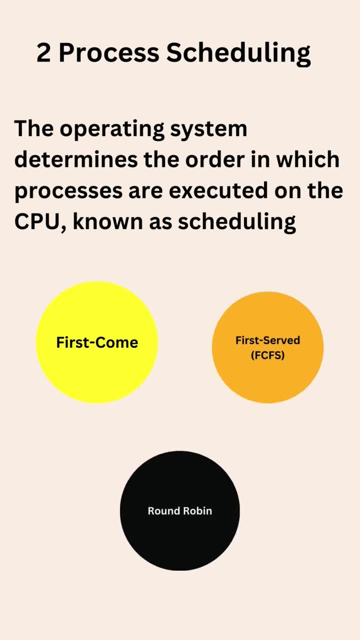 first-served FCFS or round-robin are used to manage process execution. 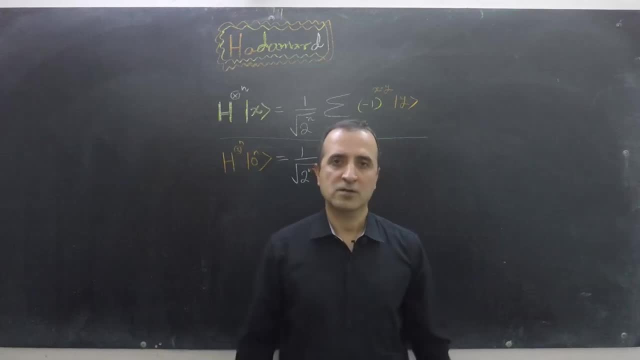 In the last two videos we have learned that how to use Hadamard gate on a single qubit and how to extend Hadamard gate to use on multiple qubits. In this video we will learn that from where such equations come Basically, when we are. 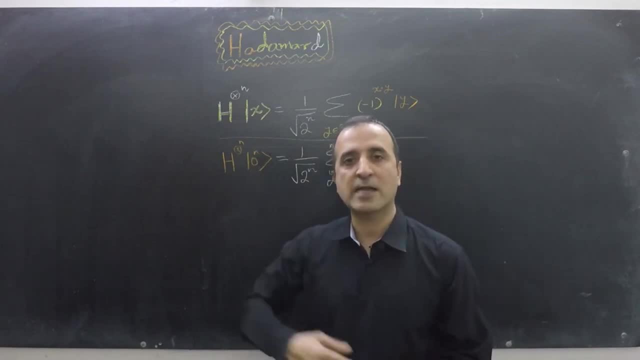 dealing with Hadamard gates and we want to apply Hadamard gate on any n qubit. we just write either this equation or this equation directly and some of the students are not able to understand that, what happened, from where these equations come. So in this video I will try to basically drive these equations. So let's. 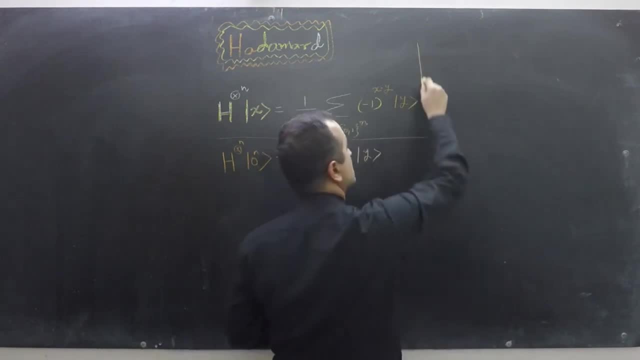 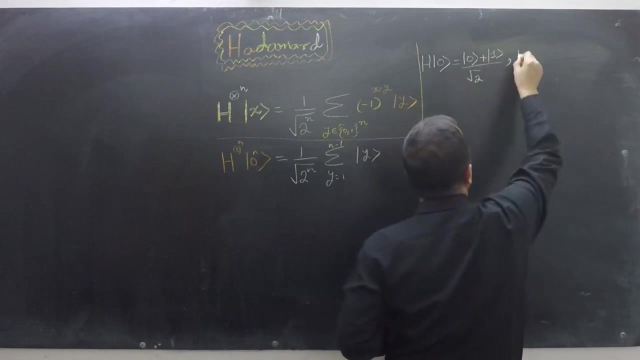 start. So let's start from this part of the board first. So we know that when we apply Hadamard gate on ket 0, then my answer is ket 0 plus ket 1 divided by square root of 2.. In contrast, if I apply Hadamard gate on ket 1, then my answer is ket 0 minus ket 1 divided by. 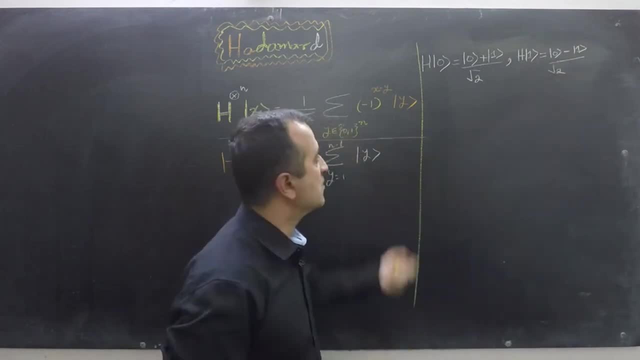 square root of 2.. In the first step I have to combine these two formulas in one formula. I can combine them by saying that Hadamard gate being applied on X, where X could be either 0 or 1.. So then this rh education becomes että 0.. So we do the same thing with 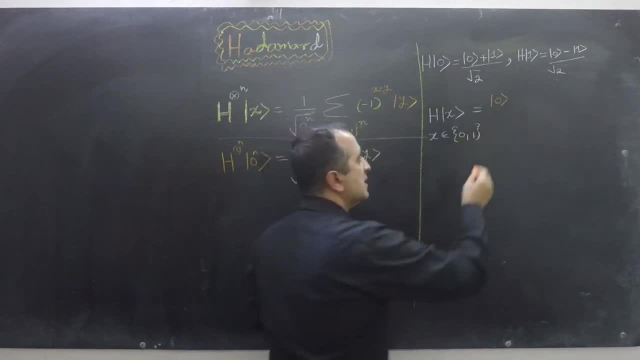 arti 1 is t. so I'll say: getting zero is ket 0, because ket 0 is common in both of those formulas. so I can школa, oh, so I can write: get zero as it is, and then it will be Garrett 0 as it is, and then it could be: